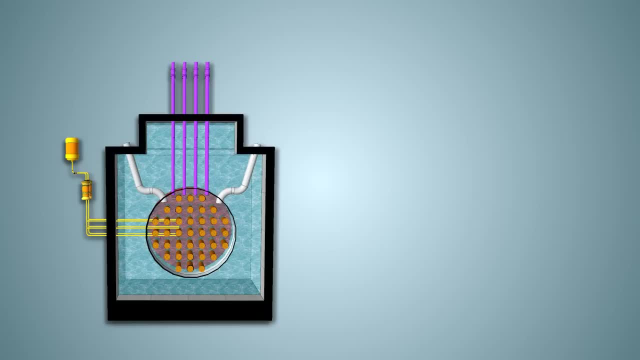 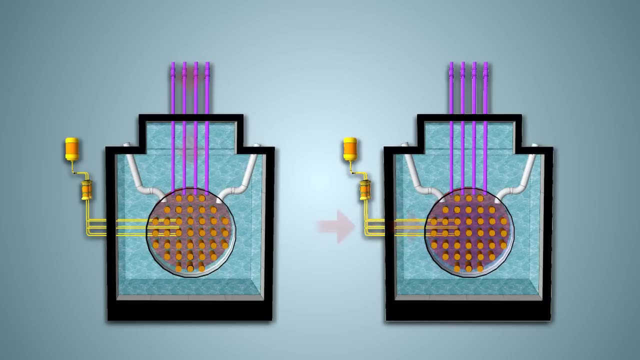 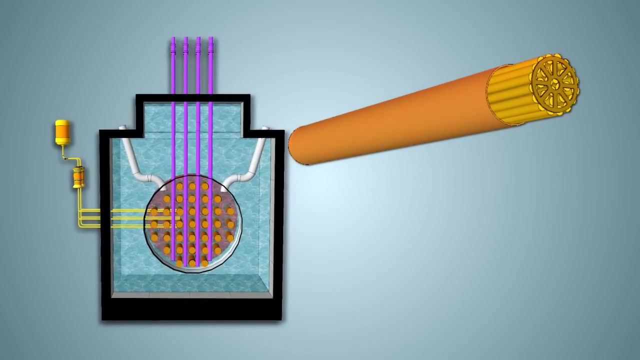 If on-site power is also lost for some reason, shutdown systems are activated automatically and the reactor stops within two to three seconds. CANDU reactors have two independent fast-acting shutdown systems that work without power or worker intervention. Even though the reactor is shut down, the fuel inside the reactor continues to produce heat and needs to be cooled. 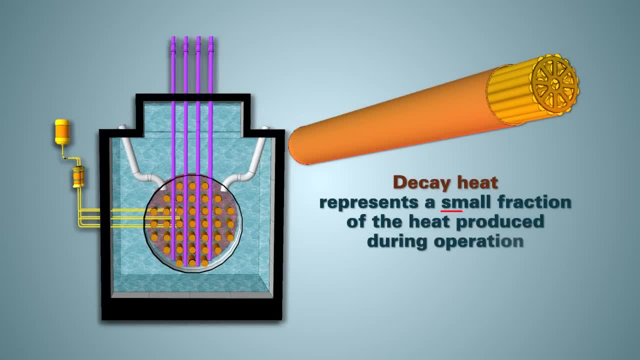 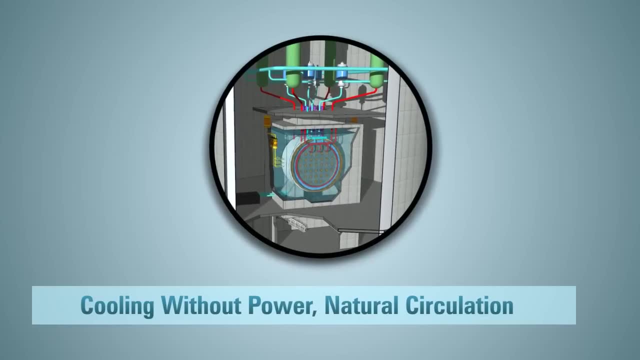 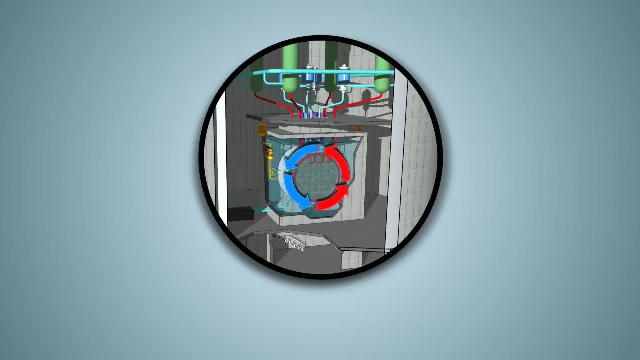 This heat is called decay heat and represents a small fraction of the heat produced during normal operation. This is a small fraction of the heat produced during normal operation. This is a small fraction of the heat produced during normal operation. To reduce this heat, natural circulation takes over when the pumps that normally push the coolant through the heat transport system lose power and stop working. 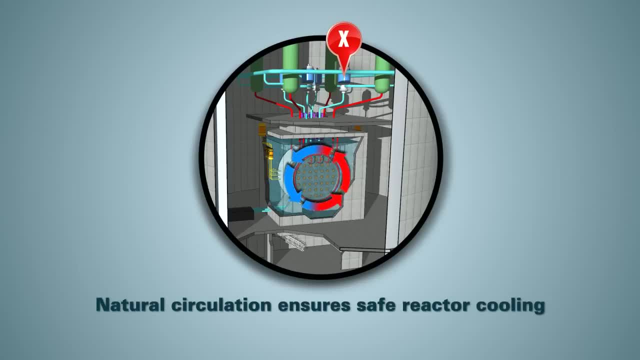 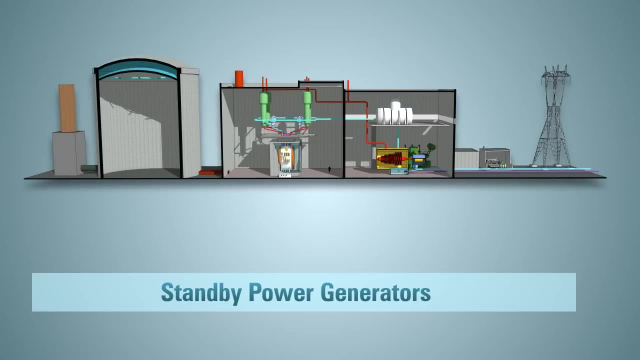 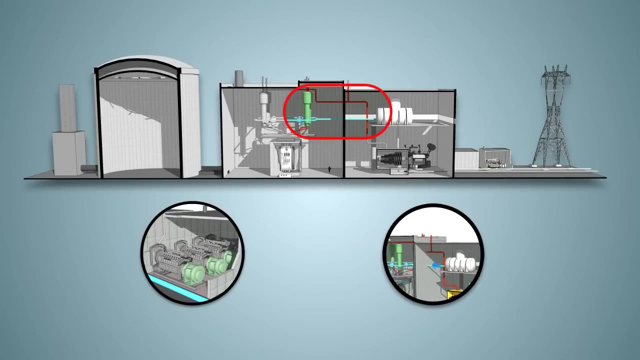 For natural circulation to continue over time, the steam generators need to be filled with cool water. Stand-by power generators operate pumps that provide this cool water to the steam generators. Stand-by power generators operate pumps that provide this cool water to the steam generators. 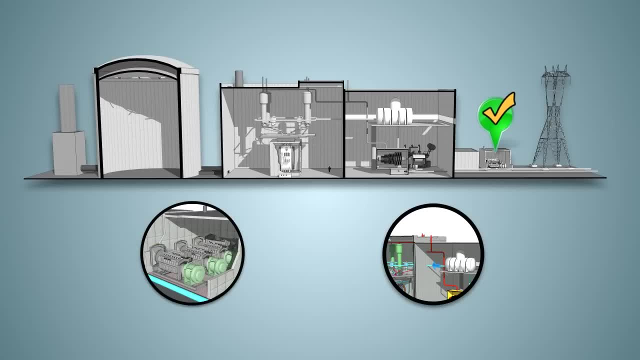 A nuclear power plant needs one or two standby power generators, depending on the size of the plant. A nuclear power plant needs one or two standby power generators depending on the size of the plant, But, as a precaution, all plants in Canada have three or four available. 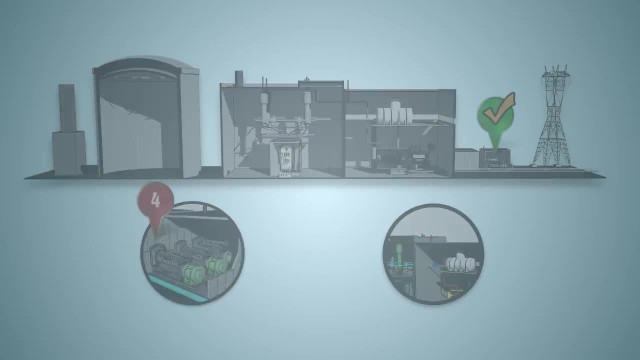 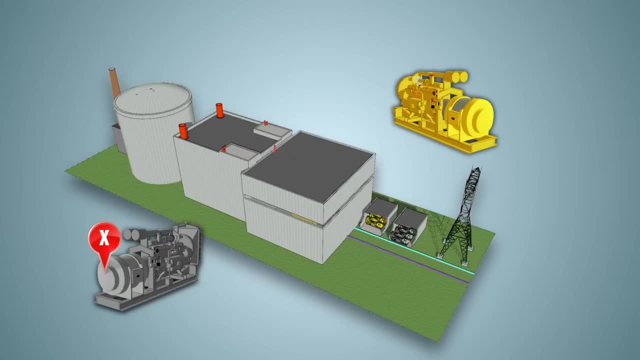 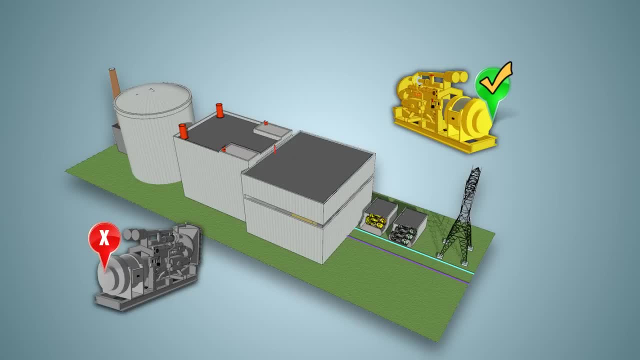 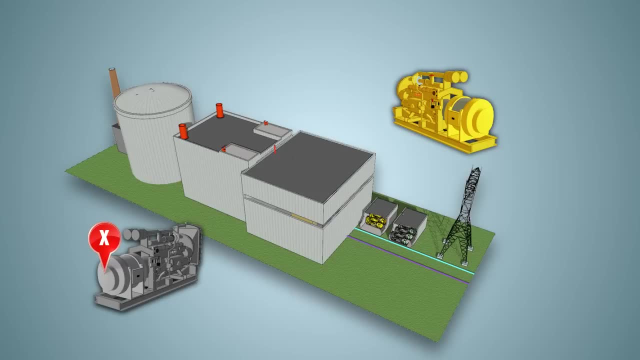 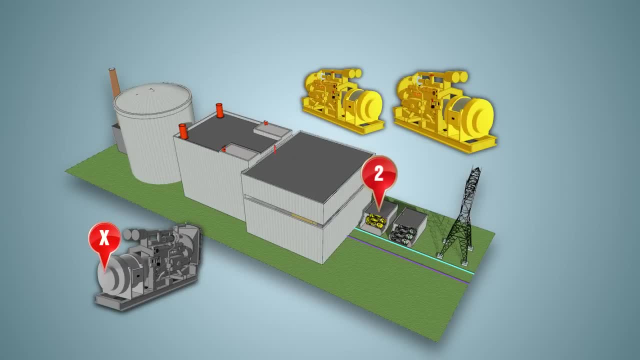 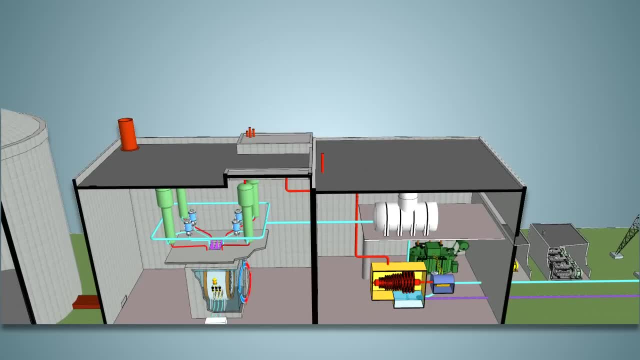 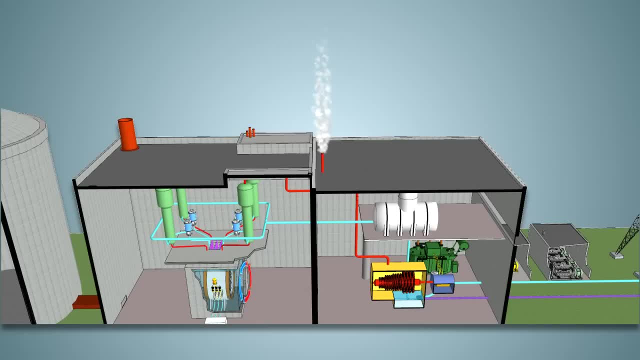 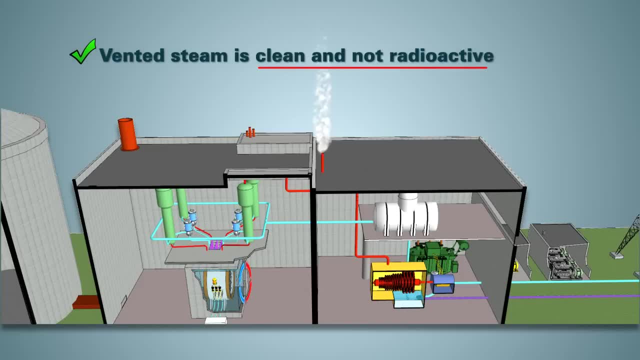 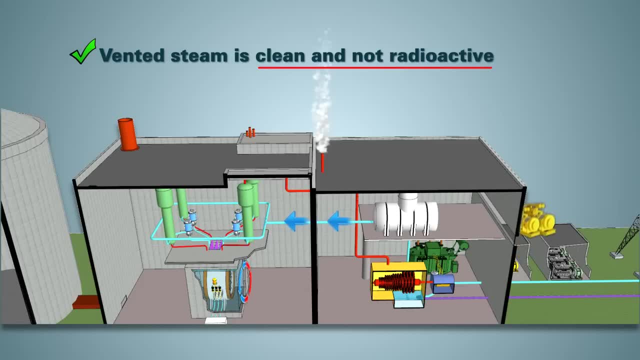 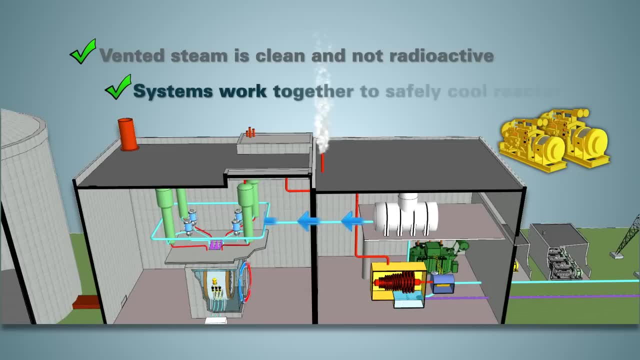 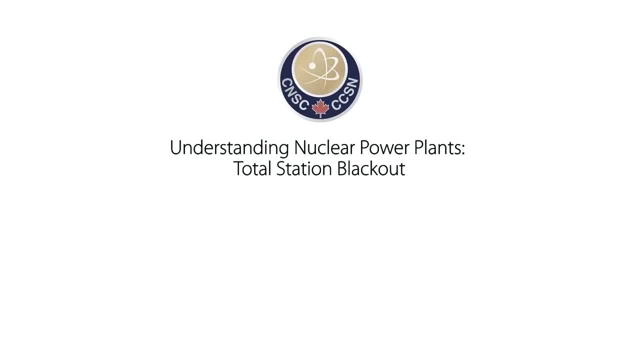 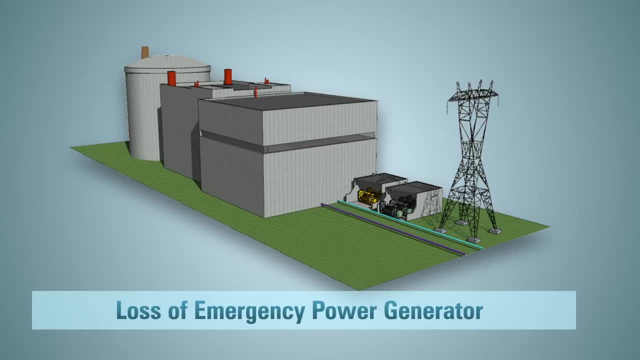 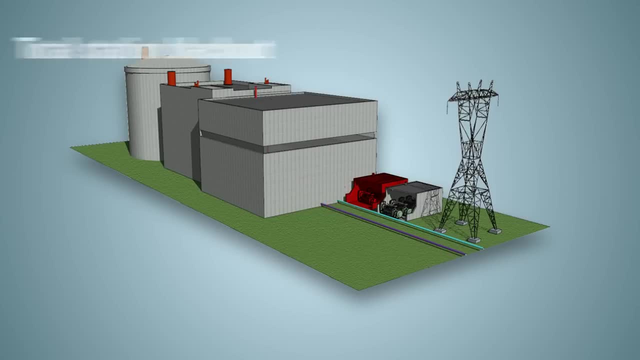 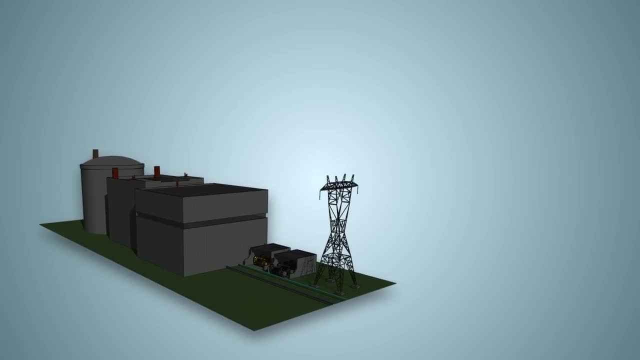 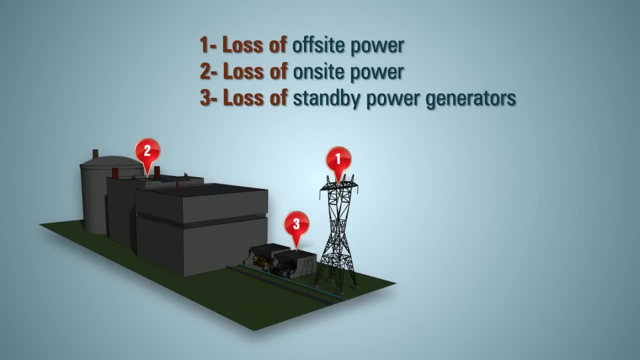 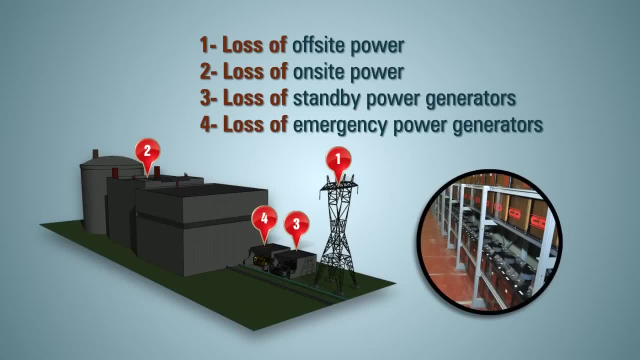 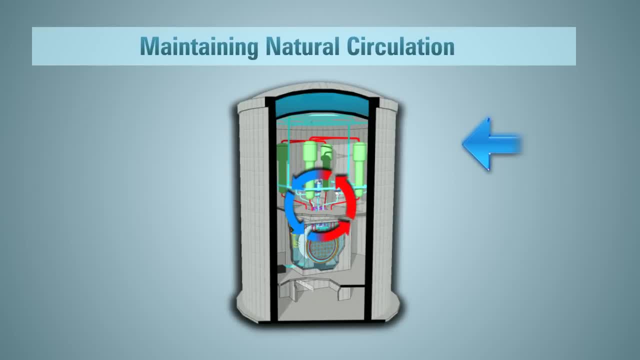 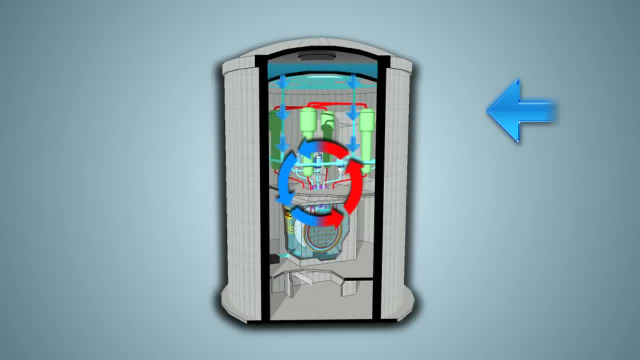 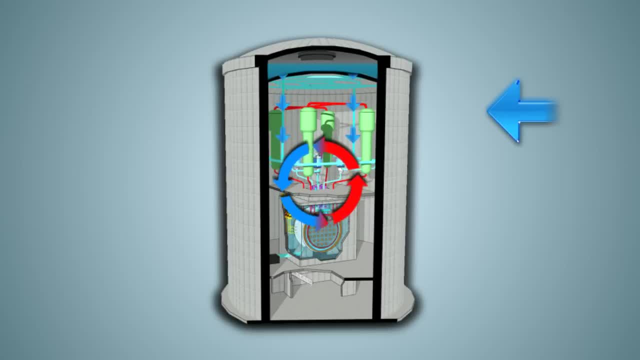 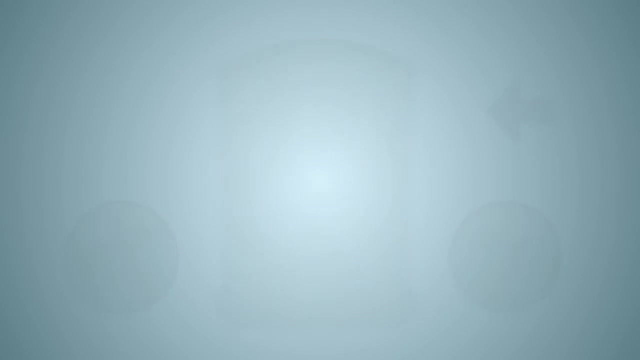 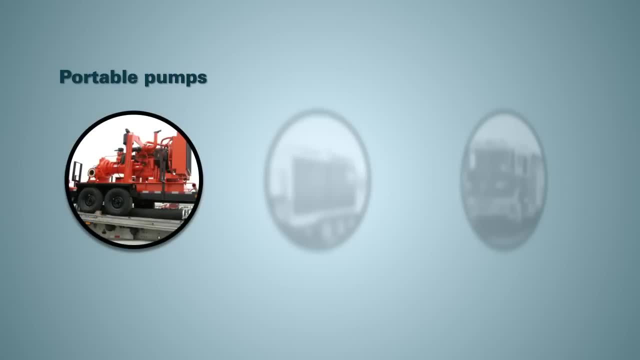 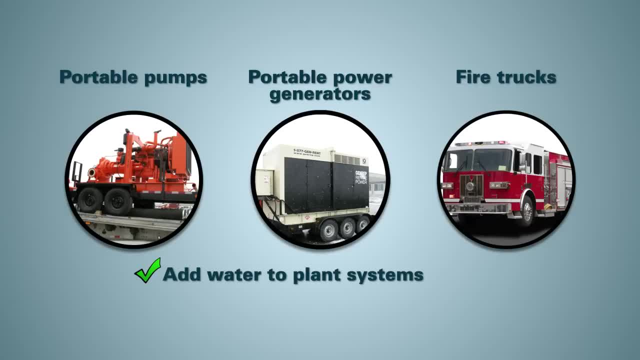 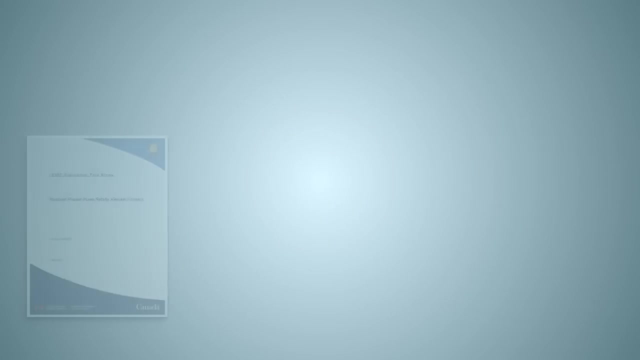 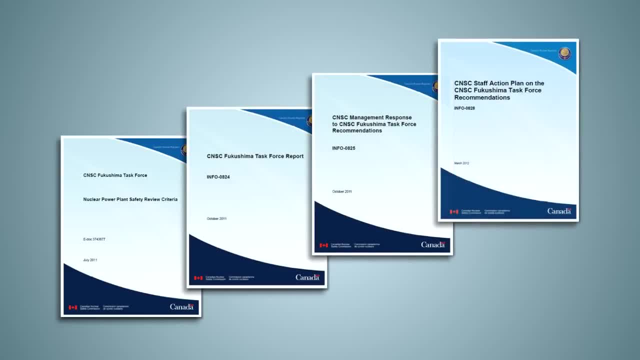 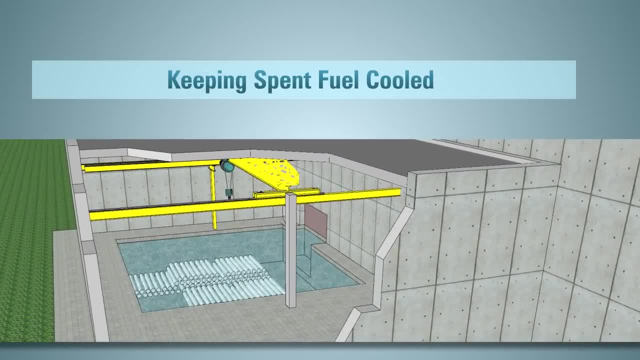 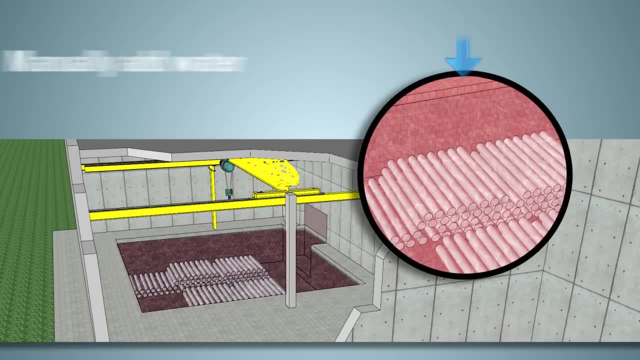 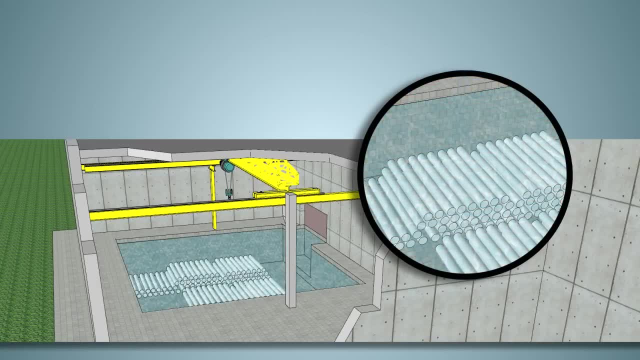 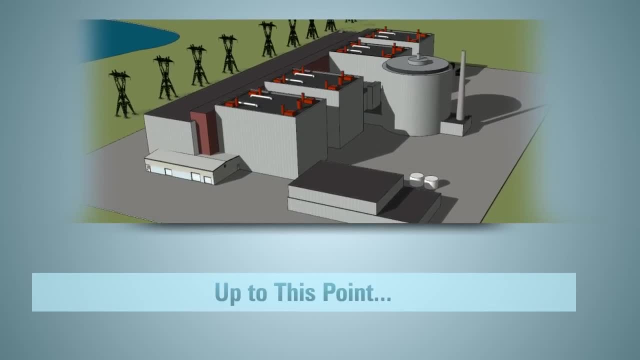 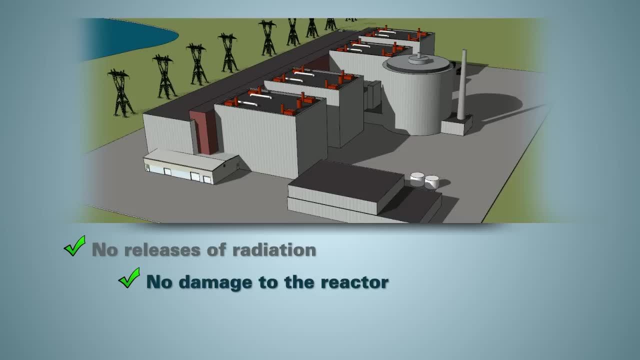 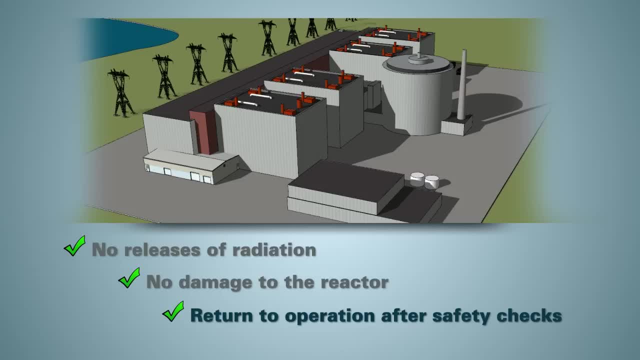 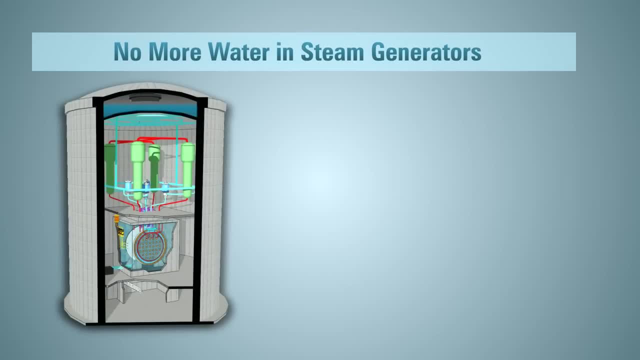 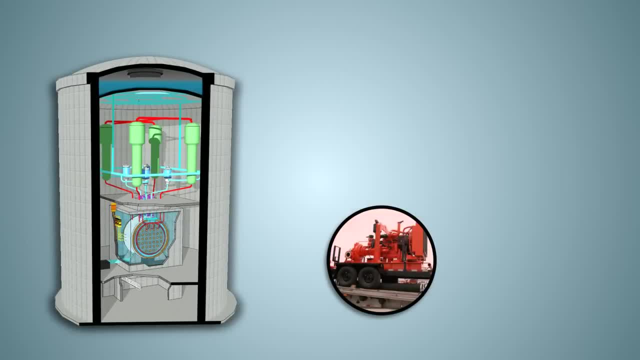 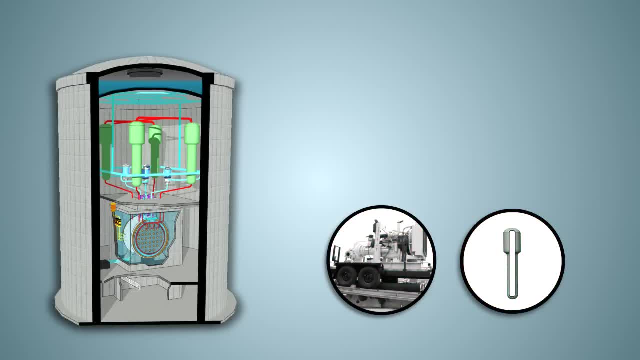 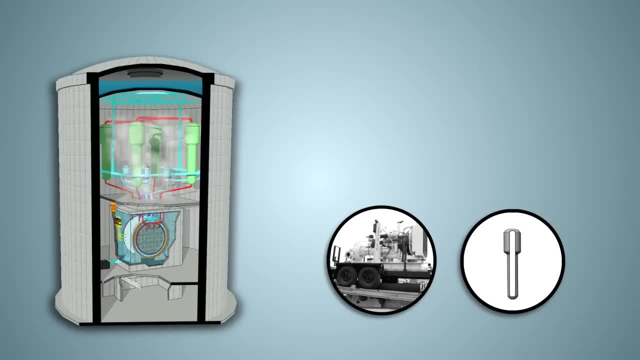 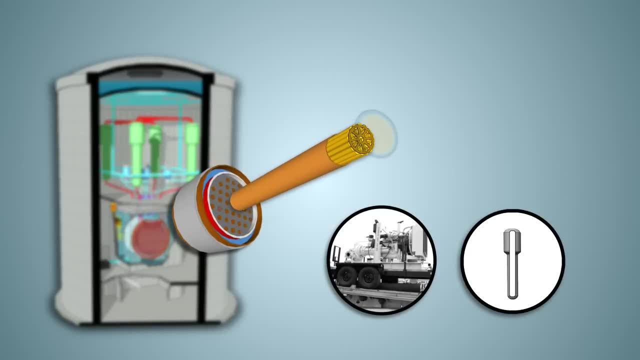 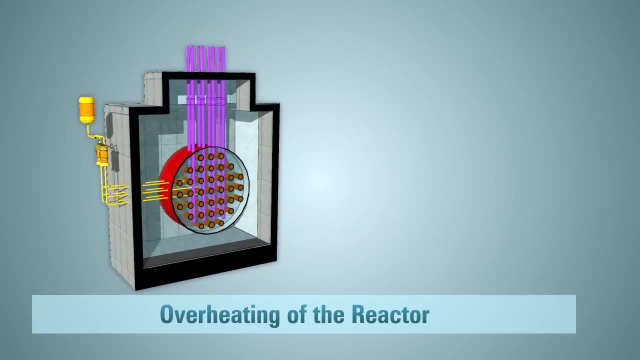 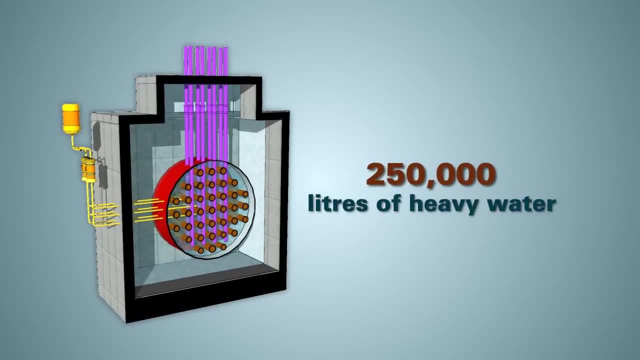 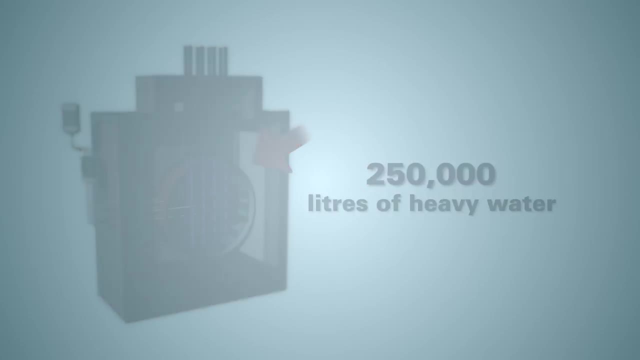 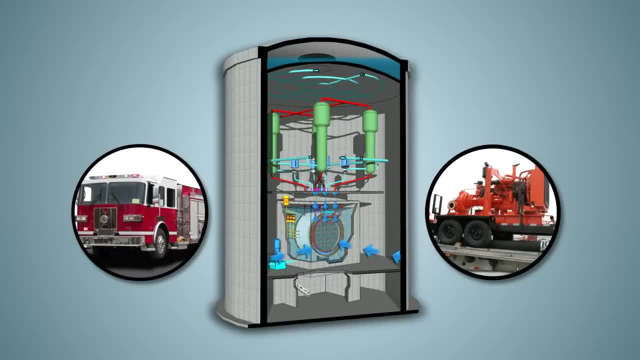 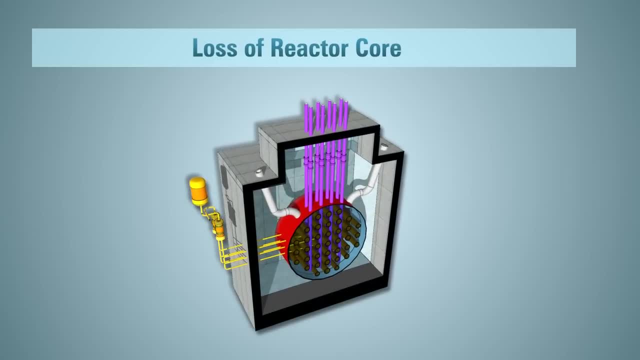 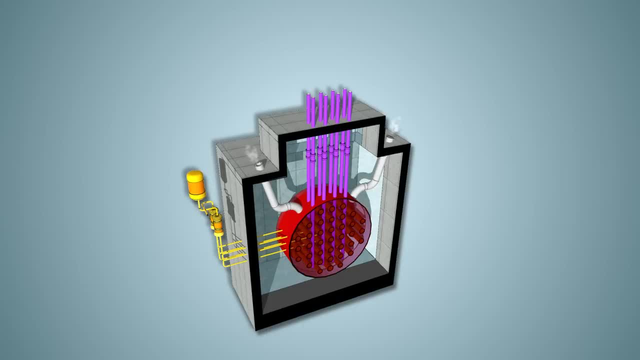 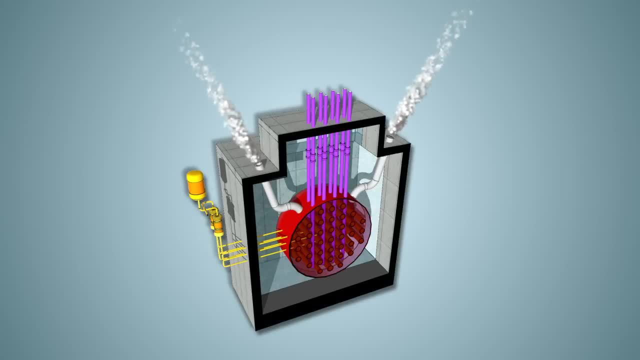 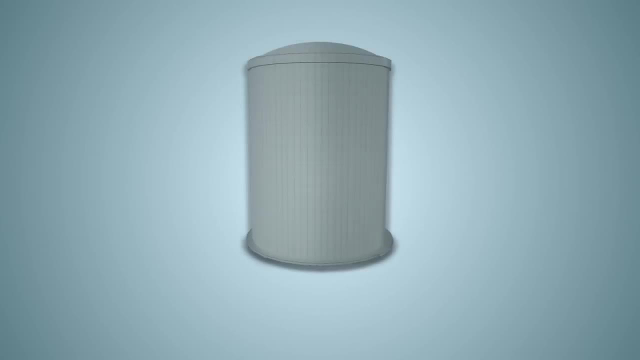 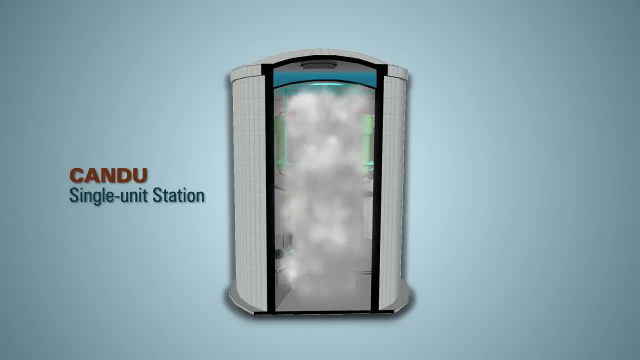 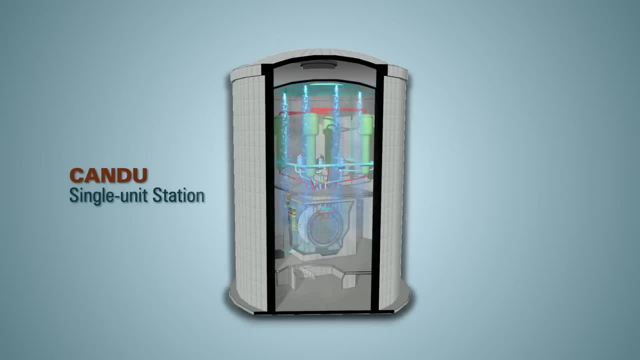 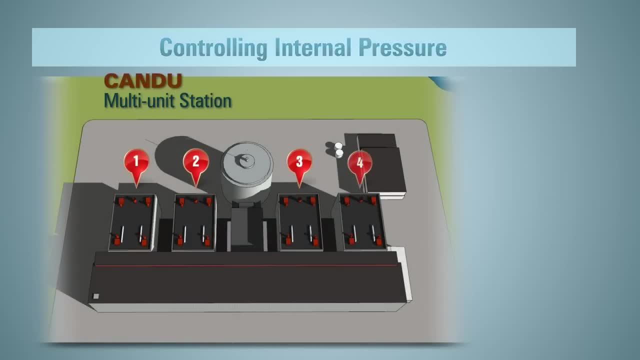 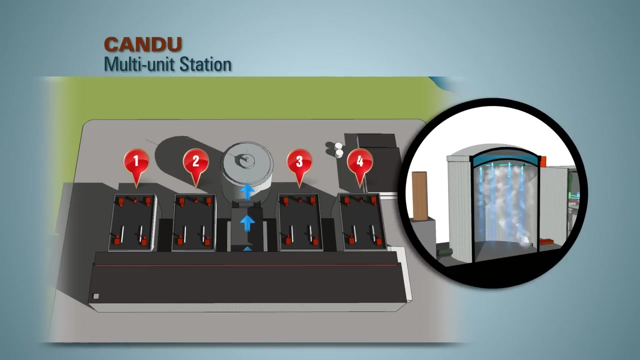 If, for some reason, standby power generators stop working. emergency power generators are then used In a multi-unit station. pressure is lowered by releasing steam and hot gases from the reactor building to the vacuum building. The vacuum building is a structure specifically designed to quickly and safely lower pressure inside the reactor buildings. 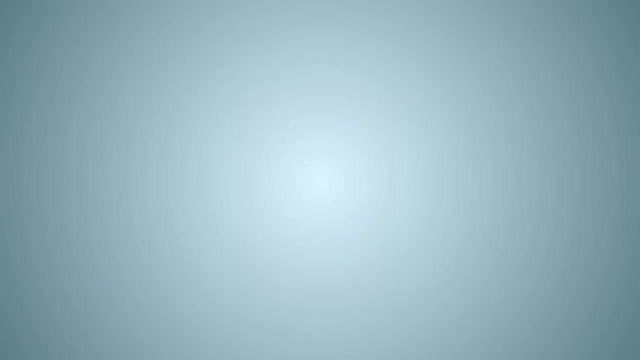 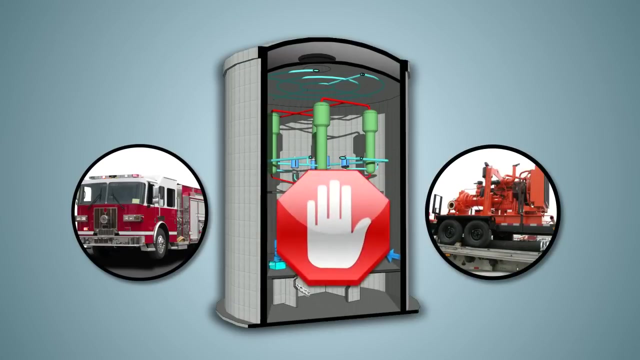 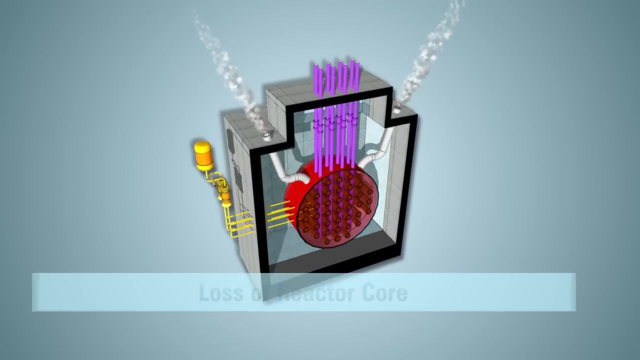 Both systems work without power. Again, supplying water to the calandria using emergency equipment such as fire trucks would stop the accident. Assuming the accident is not stopped, all remaining heavy water evaporates, The exposed fuel begins to melt and the reactor core starts to collapse inside the calandria. 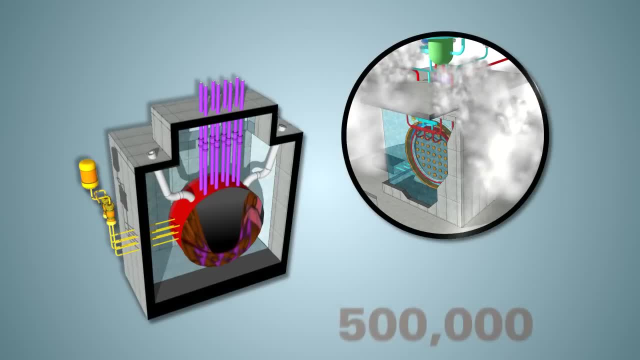 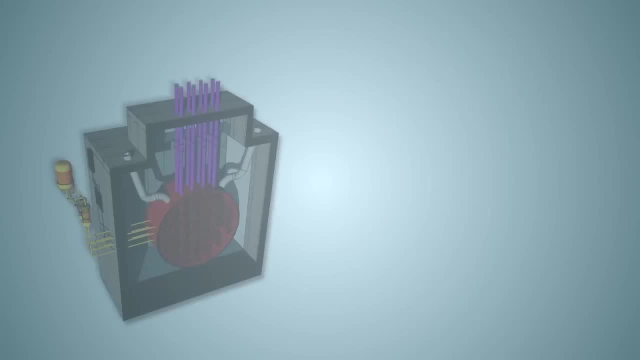 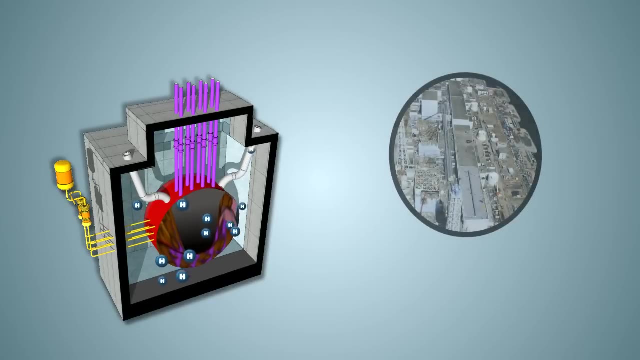 The vault that holds the calandria also holds about 500,000 litres of additional water. That water now starts to heat up. When nuclear fuel melts, it creates hydrogen, an explosive gas. You may remember this from the events in Japan. 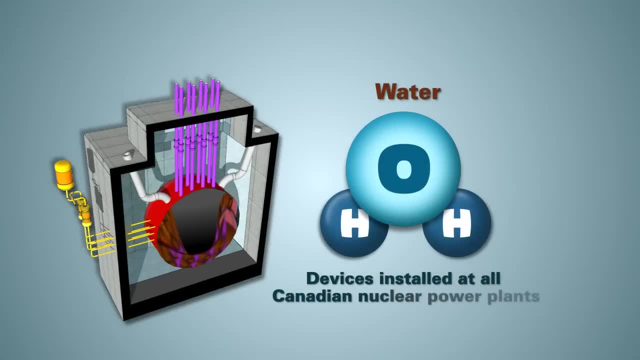 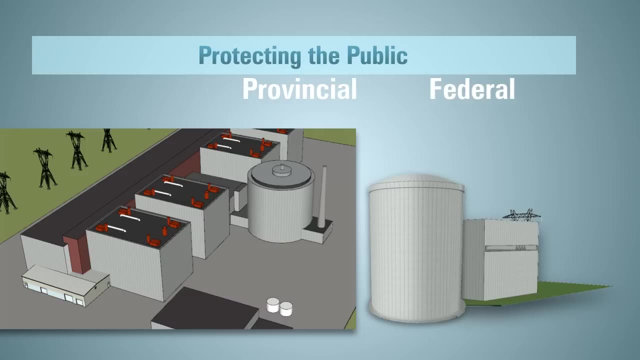 In Canada, special devices that convert the hydrogen to water have been installed at nuclear power plants to reduce the risk of explosion. These devices also work without power. At this point, federal, provincial and municipal emergency plans have been activated To protect the public. health officials have evacuated the area.